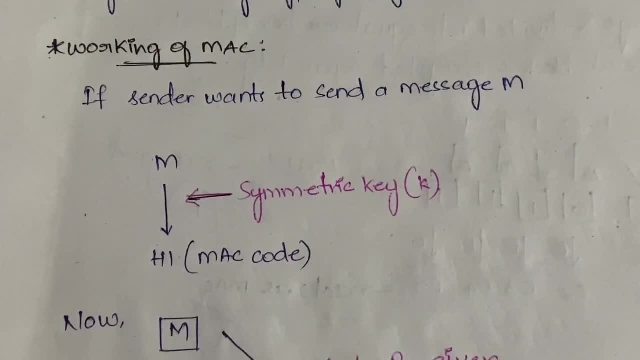 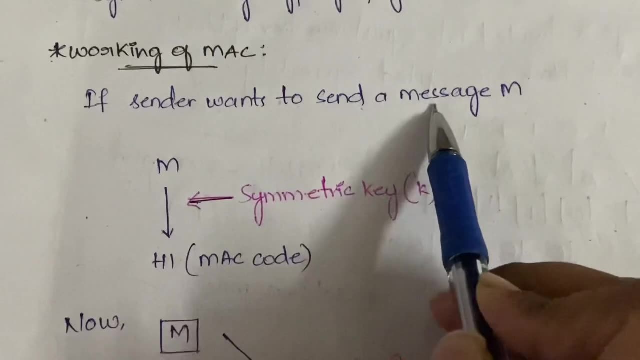 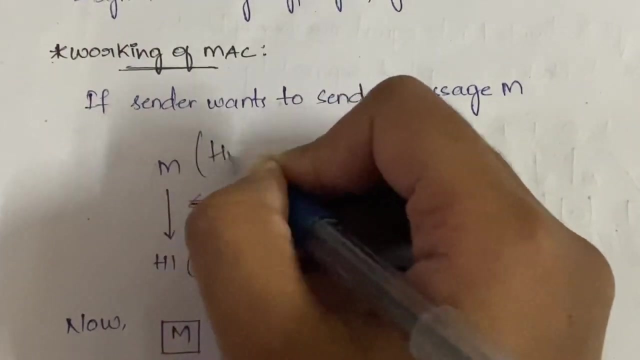 us see what is the working of mac and after working of mac, we will also understand what is the significance. that is, we can say importance or benefits or advantages, whatever it is right. so if a sender wants to send a message, m right. a sender wants to send a message m. this, m could be anything. it could be hi, hello, whatever. 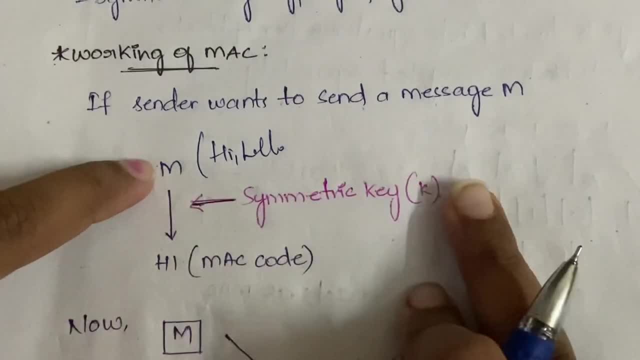 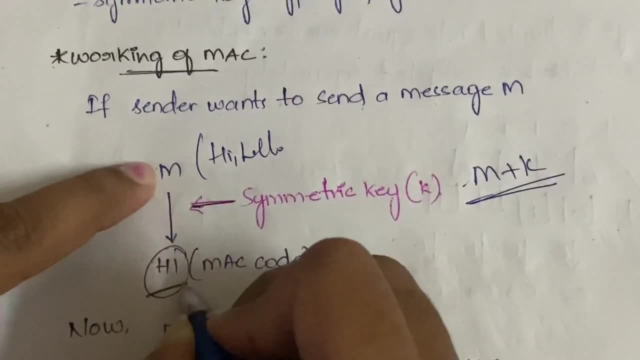 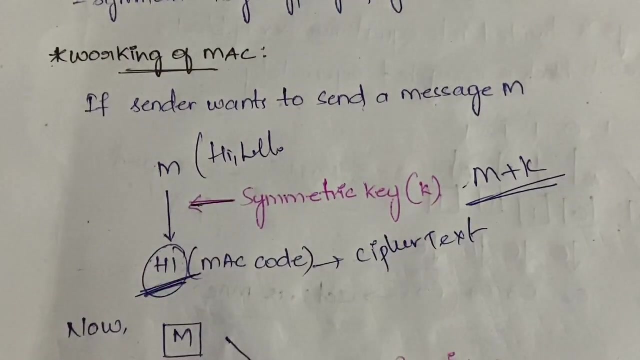 so message m plus symmetric key k got it. message m plus symmetric key k are combined together and h1 is generated. now, what is this h1? it is actually cipher text. okay, so here this h1 will act as the cipher text. h1 is nothing but the mac code message: authentication code: right. 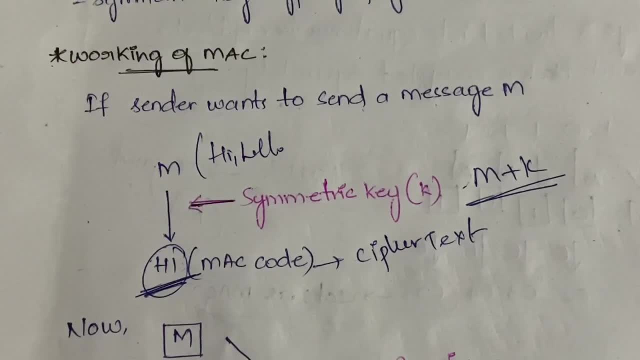 this will act as a cipher text. so in the previous video, if you have seen, we have three different types. right, we have authentication, we have mac and we have the digital signature. so, like i have done three in authentication requirements, have done three. we have three types in that. 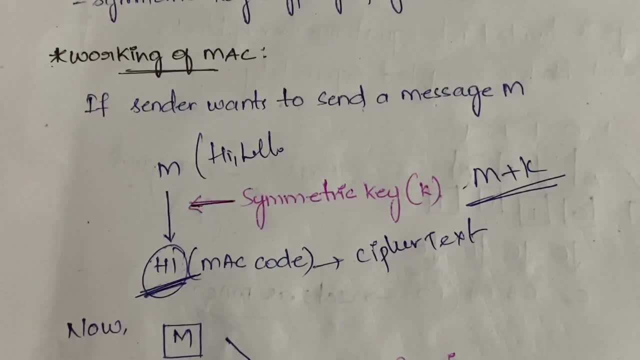 this is sorry, not digital signature, hashing authentication and mac and hashing three. we used to have right, so in that it is mac. so in mac h1 mac code is generated. this h1 mac code will act as the cipher text got it. now. what happens next is m and h1, the message and the 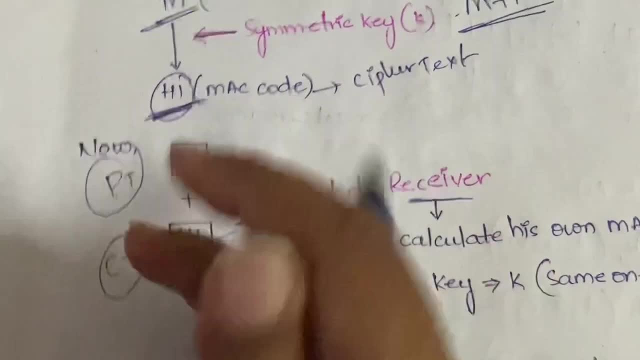 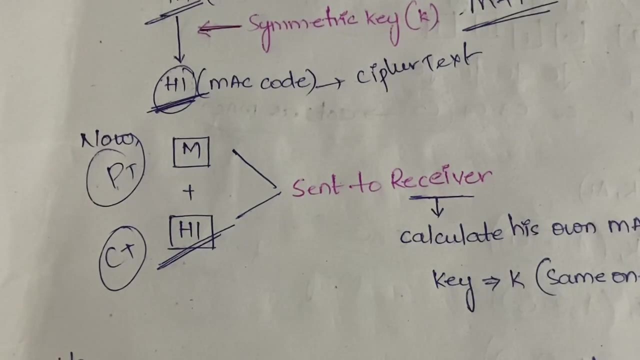 h1. that is the plain text and cipher text. you know, to understand clearly, i'm writing it as plain text and cipher text, but in exam it is better that you write message and hash code itself, because it is related to mac, right? so message and hash code, both are combined. 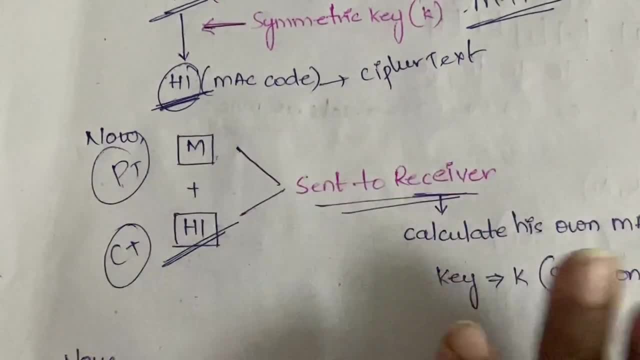 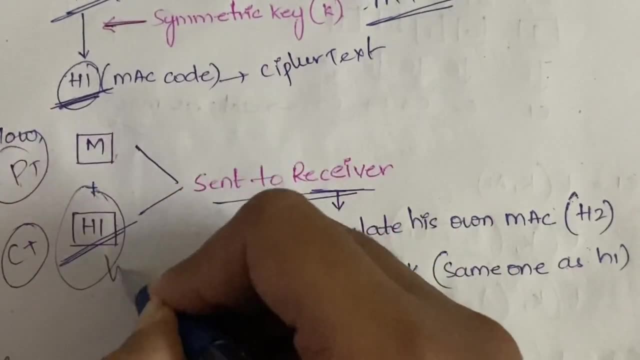 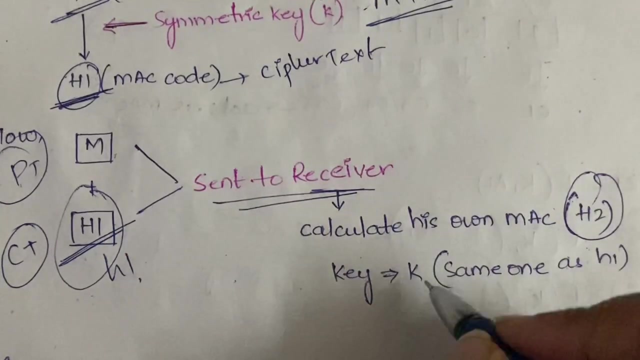 together and it is sent to the receiver. got it now. what receiver will do? receiver will also will calculate his own mac code here. what is the mac code generated on the senders? and h1, so receiver will also generate his own mac code. h2, but how? by using the k key. 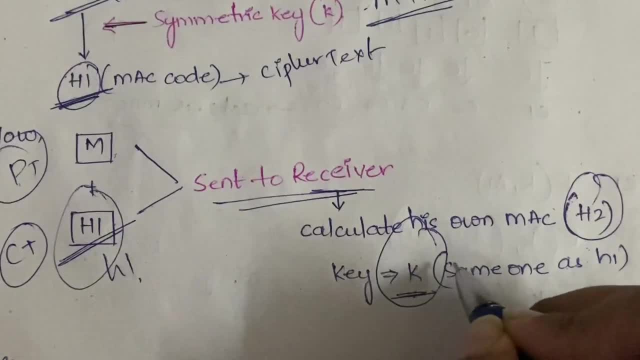 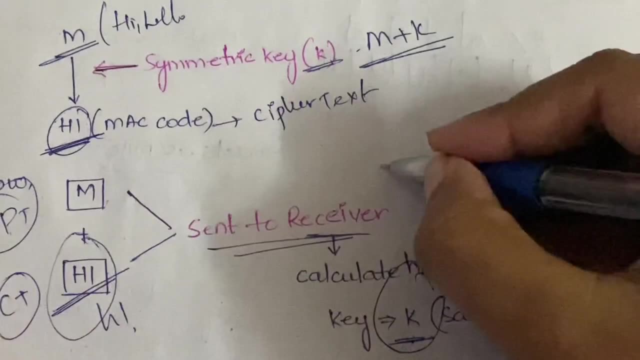 k. here the k key k is nothing but the same key we have used here. so on sender side, whichever key you are using, on the receiver side also you have to use the same key, since it is symmetric key. got it symmetric key algorithm right. so by using: 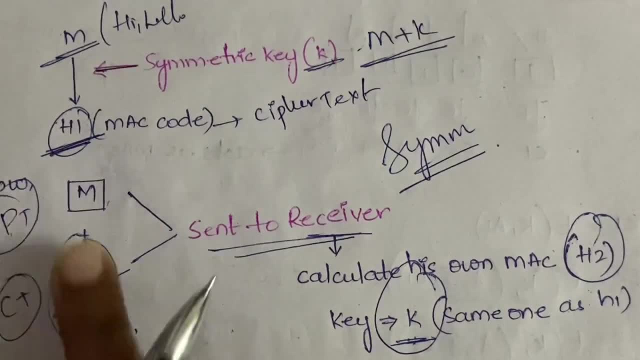 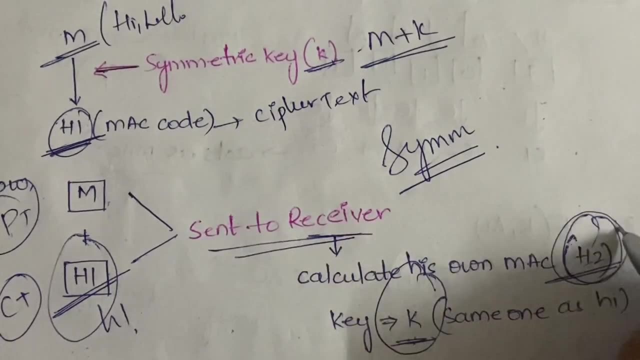 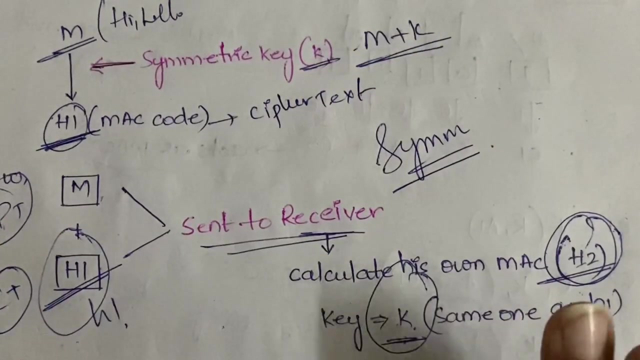 the message and the hash code. that is mac code- sorry mac code- which is sent to the receiver. the receiver will calculate his own mac code, h2 by using the key k right. since it is symmetric key algorithm, we are using the same k on both, the so same key on both. 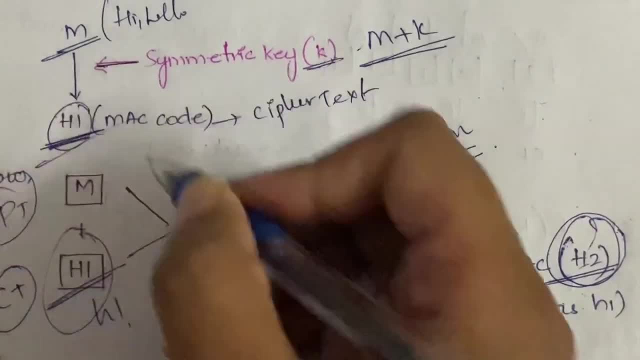 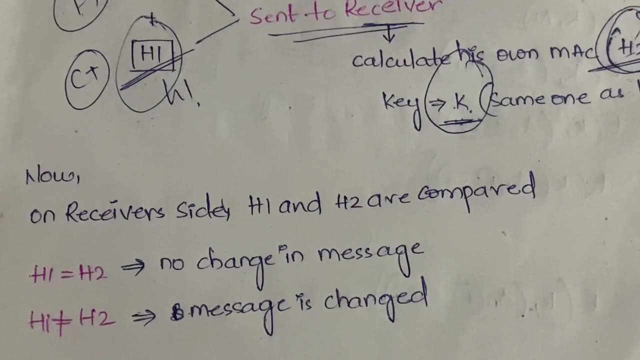 the ends. right now, h2 is generated. so here, happy h1 is generated and here h2 is generated. set now what we have to do. now you need to compare both h1 and h2. if h1 is equal to h2, then there is no change in the message. that is whatever message, suppose, you send hi to. 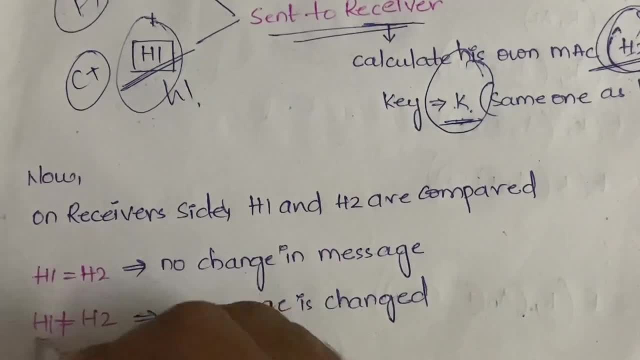 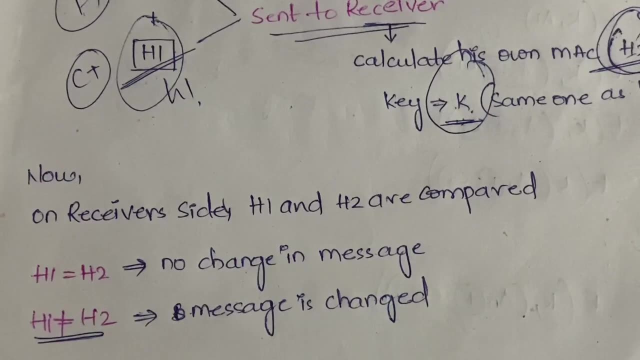 your friend. the same hi is transmitted if h1 is not equal to h2, which means the message is changed. that is, somebody has come into the middle and some attacker came and the attacker changed your message. got it? so this is about the message authentication code. very, 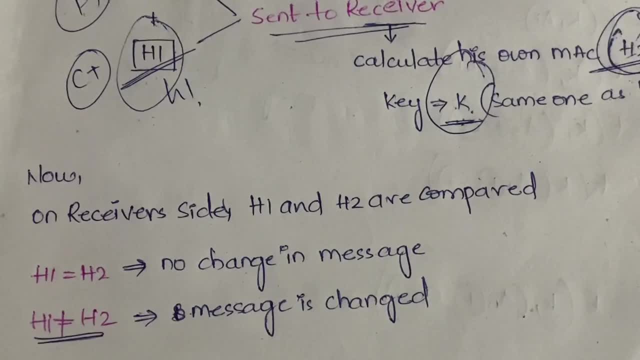 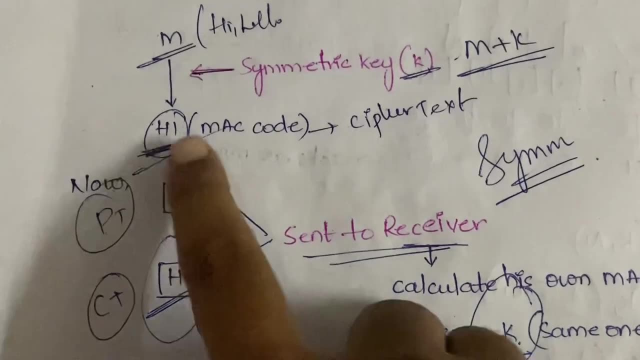 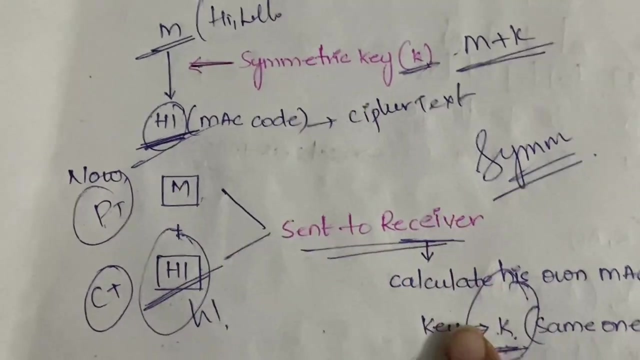 easy, very simple. so first, prior to this, watch md5 right. so in mac simple, you are using message and a key and you are generating the mac code by using. you are combining both this message and hash code and sending it to the receiver: receiver- what receiver does, he will be calculating. 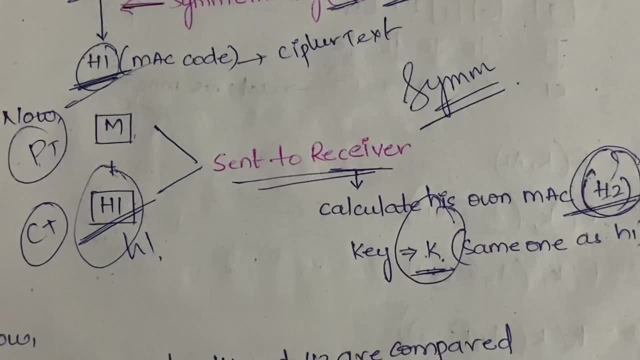 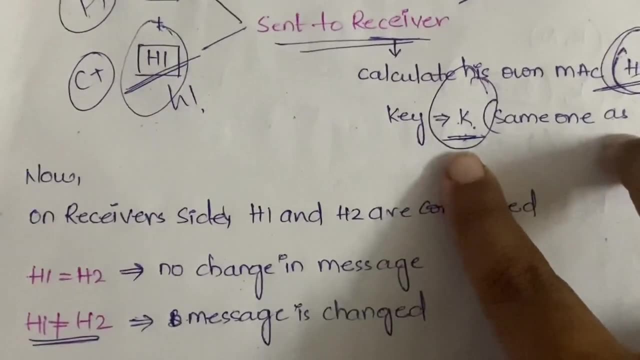 his own mac code, h2, by using several algorithms, right? and that h2 he calculates with the help of the same key which we have used here, since it is symmetric key algorithm, right? and once you get h1 and h2, you will be comparing both of them. if you get, h1 is equal to h2, which 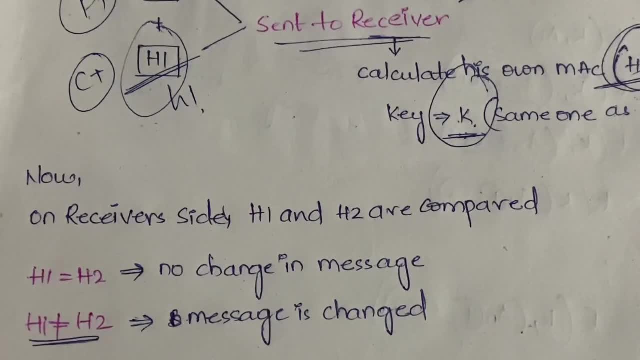 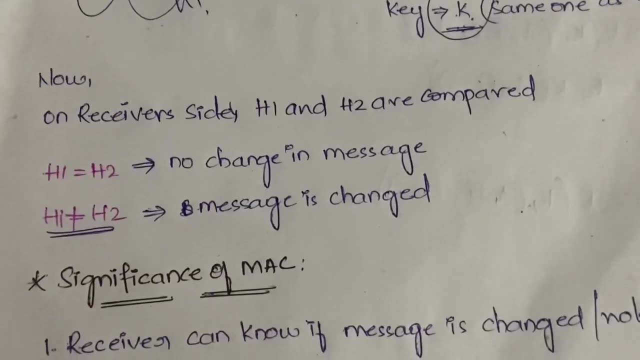 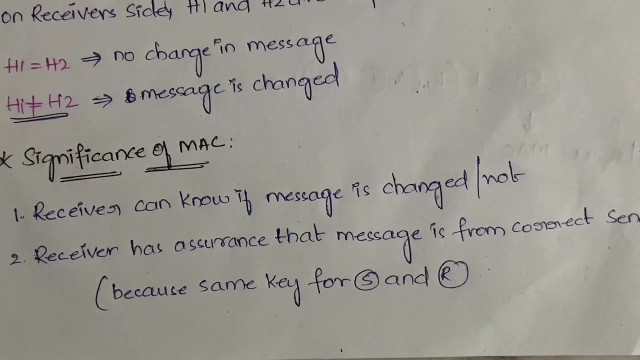 means there is no change in the message. if you don't get h1 is not equal to h2, then the message has been changed. somebody came into the network and changed the message. got it now. let us see what is the significance of mac. now moving to the significance of mac so receiver can know. i'm sorry if the message is changed or 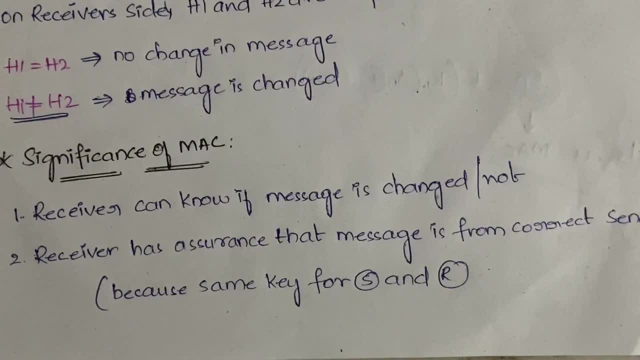 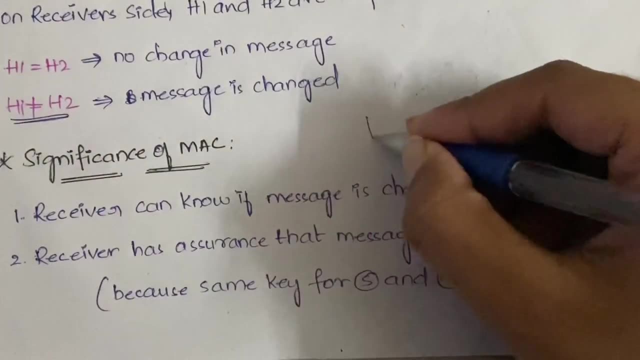 not, that is, whether the same message which i have sent is transmitted or there is change in the message. that receiver can know how by observing this hash, if h1 is equal to h2, same. if h1 is not equal to h2, changed. that's the same thing.